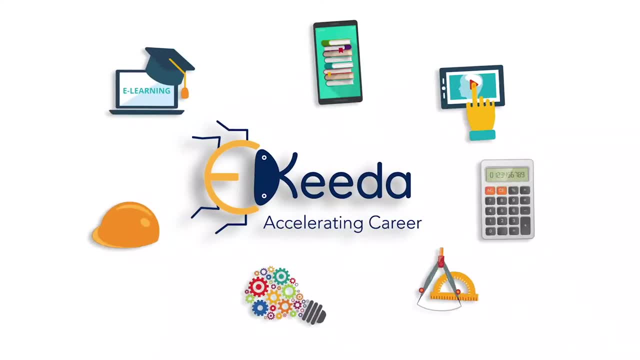 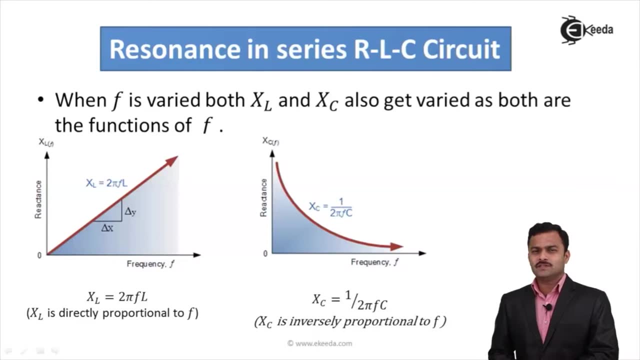 Hi, friends, in this video we are going to see the most important phenomenon in series RLC circuit and that is resonance. So resonance is nothing but that condition where total voltage applied and current flowing through the circuit will come in phase. So resultant circuit will be like a resistive, even if inductor and 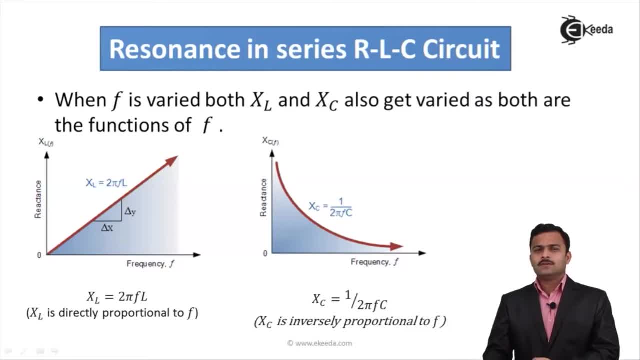 capacitor is present. Let's see how. So we have seen inductive reactance is given by 2 pi FL. So if I check this, it is directly proportional to the frequency. So if you plot, you will get a straight line passing through a origin like this: 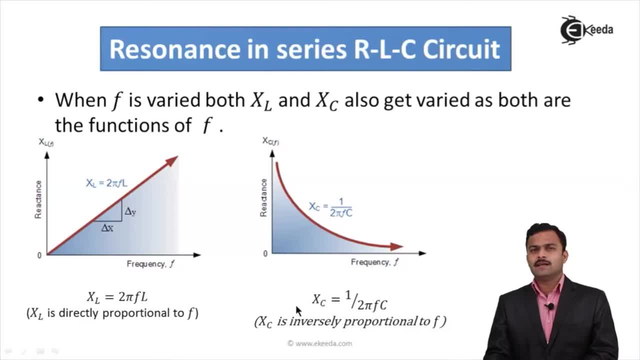 Same way, capacitive reactance is given by XA equal to 1 upon 2 pi FC, So it is inversely proportional to frequency. So if I plot I will get a rectangular hyperbola like this. Now suppose in a series: 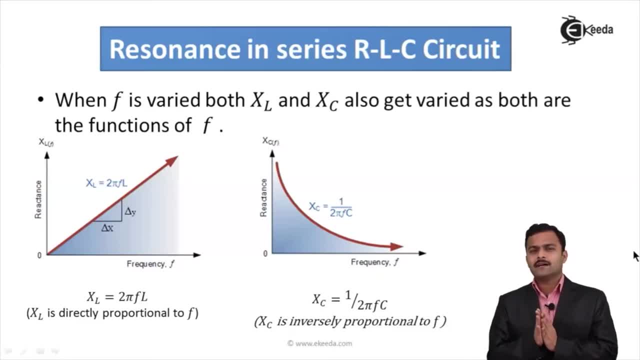 RLC circuit. both these elements are present and I am having a variable frequency source. So if I keep on changing the frequency XL and XC, both will vary in this manner. One point will be there where both XL and XC will be same. See over here. I am varying the frequency. XL is varying. 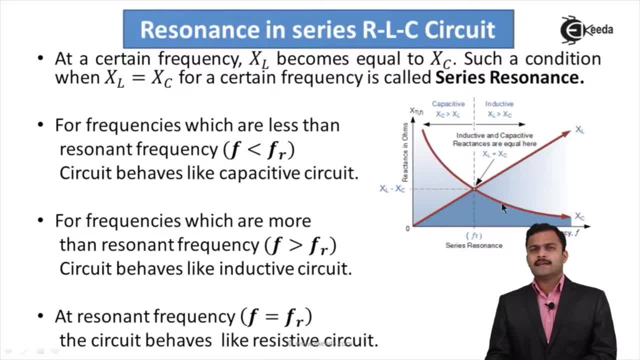 like this: XC is varying like this. So there is an intersection over here where I can say XL and XC, both are equal. So what will happen at that point? At that point, the effect caused by inductor will be nullified by effect caused by capacitor. Hence it will be like a 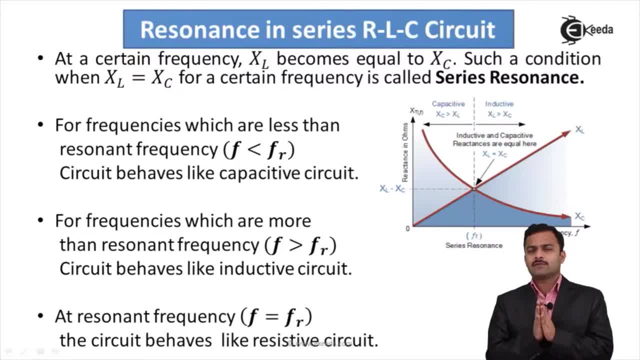 redundant. so L and C effect will nullify each other. so only passive element left is a resistance alone. so capacitor and inductor will act as a redundant, leaving behind only resistive circuit. so at certain frequency xl becomes equal to xc. such condition is called as series resonance. 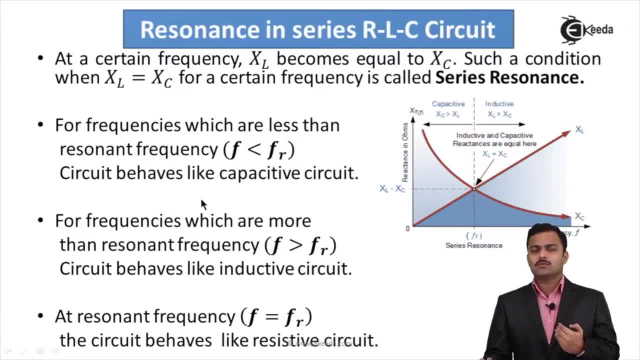 so what happened before series resonance and what happened after series resonance? let's check it for frequencies which are less than resonating frequency. resonating frequency is nothing but that frequency where resonance occurs. so before resonating frequency, if you check the graph, xc is have higher values compared to xl. so capacitive nature of circuit will be illustrated. 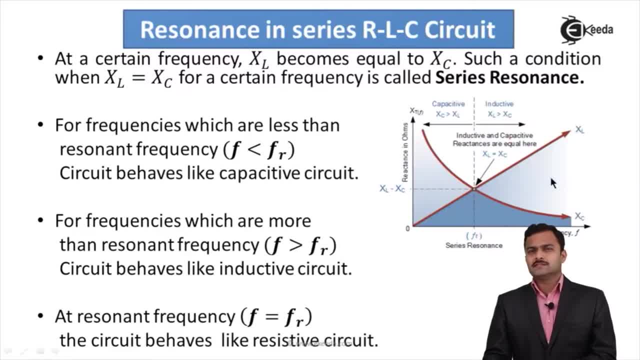 now, beyond this, the resonating frequency- i can say xl is greater than xc. circuit- behaves like inductive circuit because L is dominating factor over C. but what happened? at resonating frequency- both xl and xc are equal circuit will be resistive in nature. now this is all about the phenomenon called as 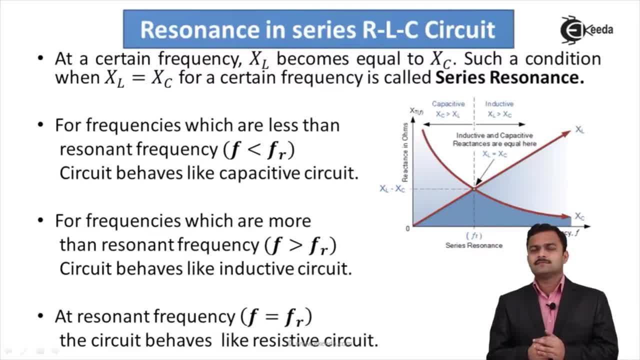 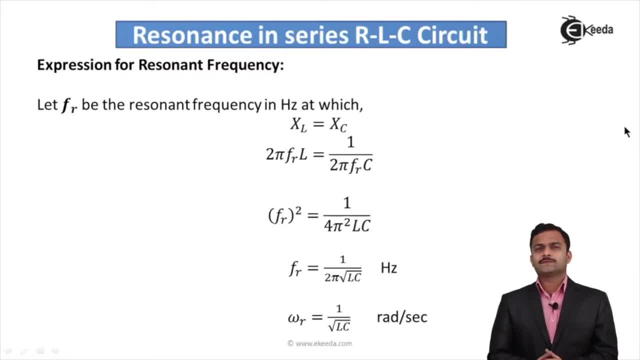 series resonance. now what are the effects on circuit because of this resonance? we will see next slide. before that let's derive the expression for resonating frequency. so let fr be the resonating frequency in hertz at which xl becomes equal to xc. so xl is given by 2, pi, f, r, L, that is equal to 1. 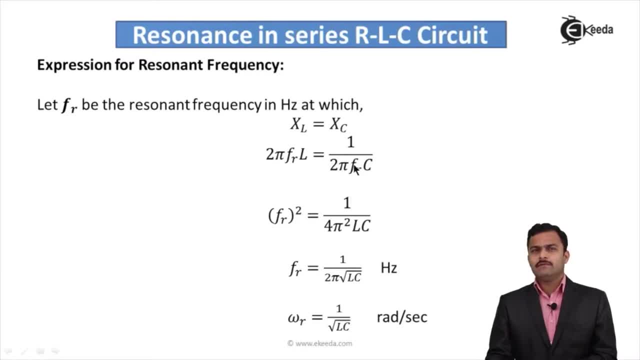 upon 2 pi f r C. if i solve i will get f? r square equal to 1 upon 4 pi square L C and taking a root i will get f? r as 1 upon 2 pi root of L into C hertz, same frequency i can write in terms of radian per second, so that is equal to omega r 1 upon root of. 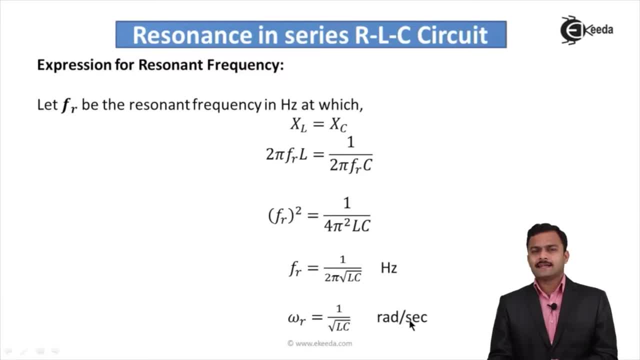 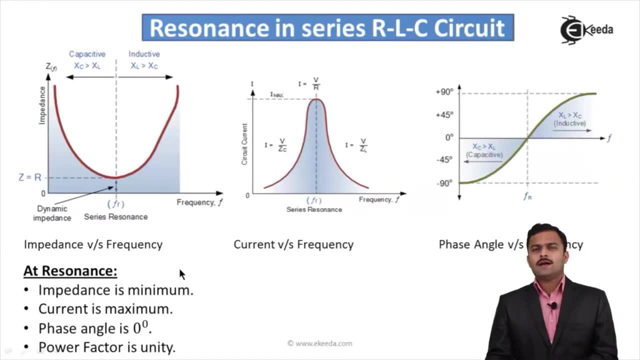 LC radian per second. what happen when resonance occurs? let's see next slide. so what happen at resonance? impedance become minimum before resonance. after resonance, impedance is given by root of R squared plus R squared xl minus xc, the whole square at resonance xl becomes equal to xc, so impedance will become. 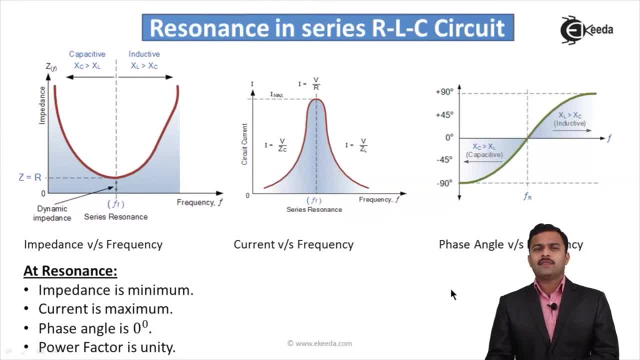 equal to resistance of a circuit only, and that will be a minimum value. so the nature of impedance versus frequency will be like this in this region as well as in this region: impedance is more, but only at resonance. it is minimum and that is equal to r. secondly, current in a series circuit. 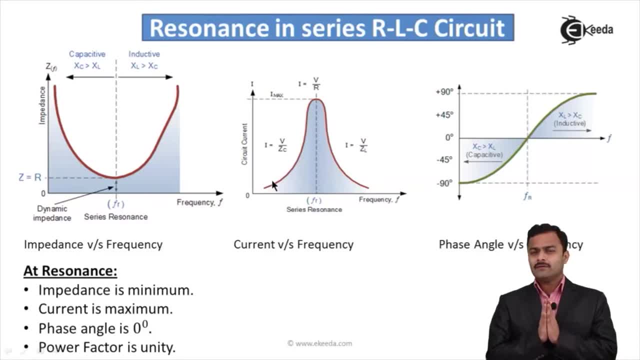 current is given by v upon z. whenever i say impedance is minimum at resonance, obviously current will be maximum. so the nature of current versus frequency will be like this: only at resonance current will have maximum value and that is given by v divided by r z, minimum, which is equal to r. so v by r will be the maximum current at resonance phase angle. 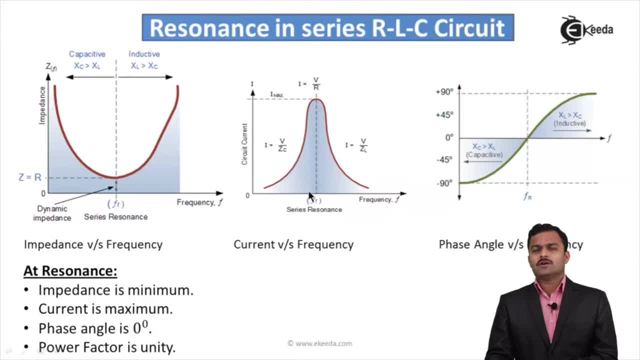 from the waveform or characteristic it is clear before. resonance circuit will be capacitive in nature. so for capacitance the angle will be negative that we have discussed earlier at resonance circuit will be. resistive angle will be zero. i'm talking about a phase angle and beyond that we have a phase angle which is equal to v by r. so v by r will be the maximum current. 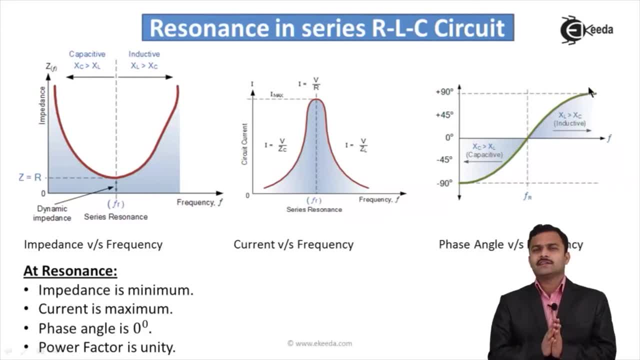 on resonance circuit will be inductive. angle for inductive circuit is positive, so the phase angle versus frequency will be like this: if i take a cosine of that, what i will get- cosine of zero degree- is one which is a maximum value of cos phi. so what happened at resonance power factor? 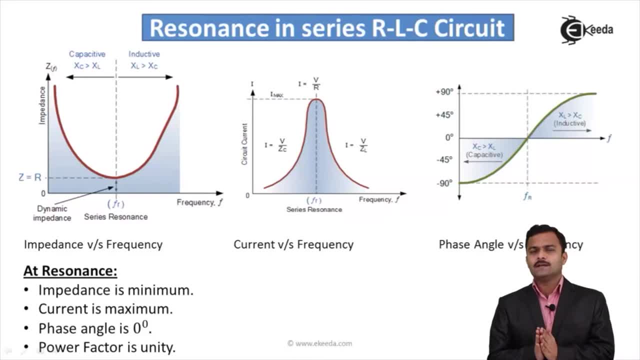 cos phi is maximum and that is equal to one before resonance. after resonance the value of cos phi is less than one. so we have to remember what are the things happening at the resonance. so i have listed it out: at resonance, impedance is minimum. current is maximum phase. 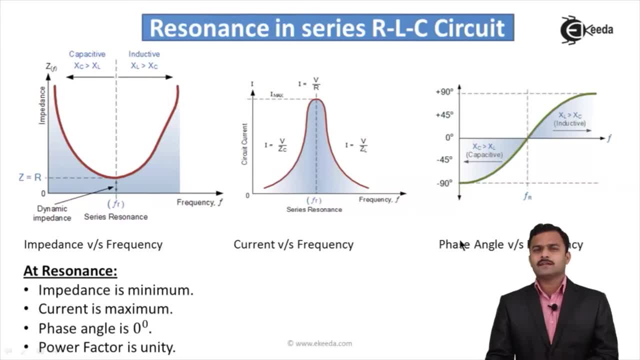 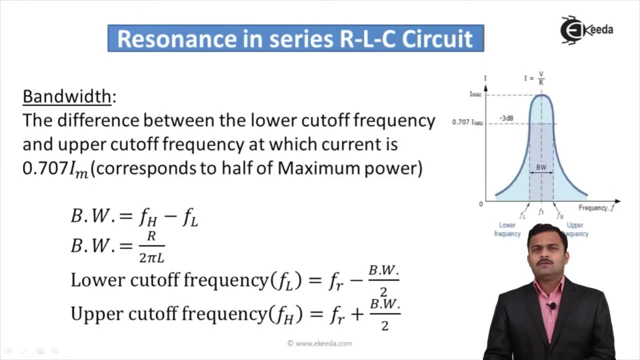 angle is zero degree at resonance and power factor is unity, which is maximum at resonance. now we have seen a resonance once current. we come to know current is maximum at resonance. obviously, power is also maximum at resonance, but here we are going to use the graph of current versus frequency to determine the most important parameter of a. 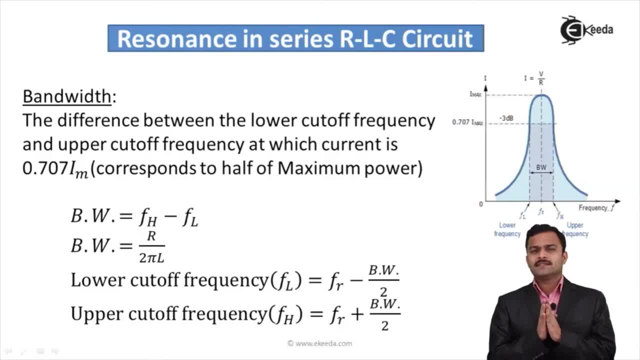 circuit and that is called as a bandwidth. bandwidth is nothing but a selectivity of a circuit to receive or give out the signal. so bandwidth is nothing but a frequency range in which signal is accepted, and those frequencies which are called as a lower cutoff and upper cutoff are nothing but frequencies at which I am getting half of the maximum power which 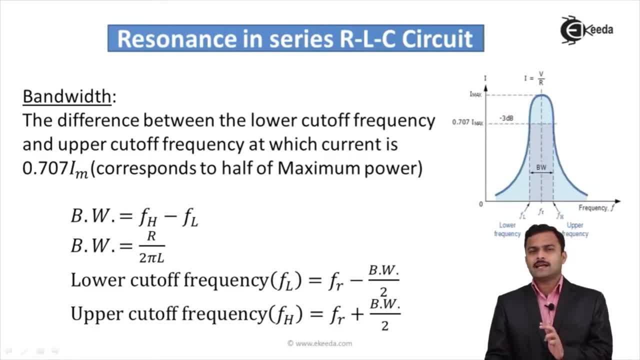 is correspond to 0.707 times the maximum current. So if I denote those values of the frequencies I will get here: lower cutoff frequency FL. upper cutoff frequency FH. and the difference between them is called as a bandwidth. So the bandwidth is nothing but the difference between the lower cutoff frequency and upper. 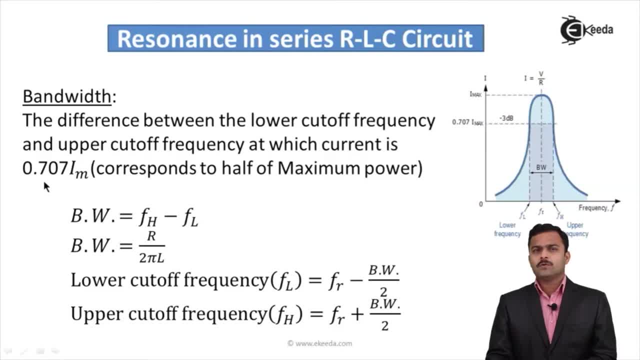 cutoff frequency at which current is 0.707 IM. IM is the maximum current and that is corresponding to maximum power. So bandwidth formula is FH minus FL. In terms of parameters of circuit Bandwidth is given by R upon 2 pi L. 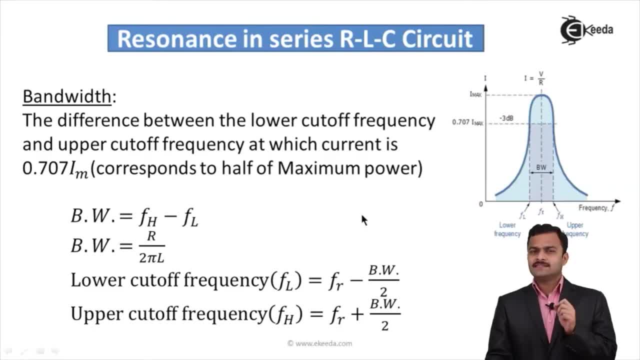 So if I know the value of resistance and inductor I can say what is the bandwidth of a circuit. If I know the bandwidth I can get a lower cutoff frequency. So lower cutoff frequency, FL, is nothing but FR minus half of the bandwidth. Same way, upper cutoff frequency, I can say FH equal to FR plus half of the bandwidth. 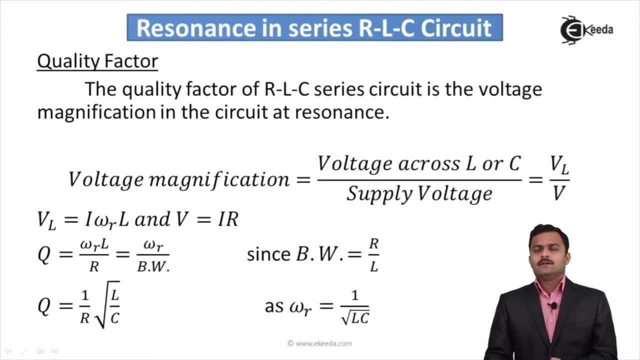 Okay, Now one more important part for a series: resonance is a quality factor. So the quality factor of a series RLC circuit is the voltage magnification in the circuit at resonance. I will explain voltage magnification. Voltage magnification is nothing but voltage across L or C divided by supply voltage. 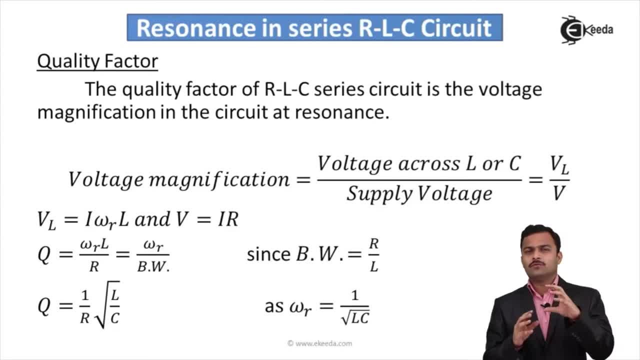 It may happen that you are supplying a voltage of 10 volts To a series RLC circuit, but voltage across inductor and voltage across capacitor you may get 100 or 1000.. So what happened over here? total voltage is 10 only and voltage across VL you may get 100 or 1000, depending upon what is the value of L and C and, obviously, resonating frequency. 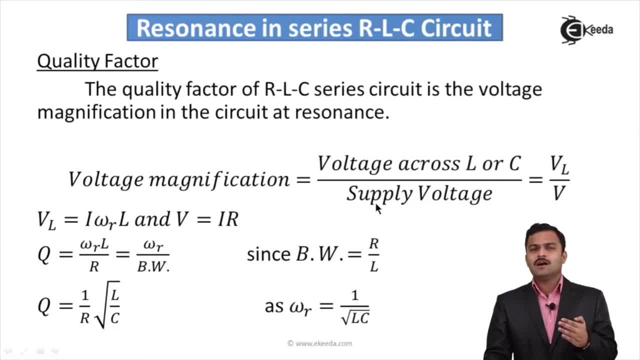 So what happened? 10 volt is getting magnified up to a higher voltage level Because of resonance phenomena. Therefore it is called as a voltage magnification, also called as quality factor of series resonance. So VL or VC at resonance is nothing but I into XL or XL resonance and XL is given by. 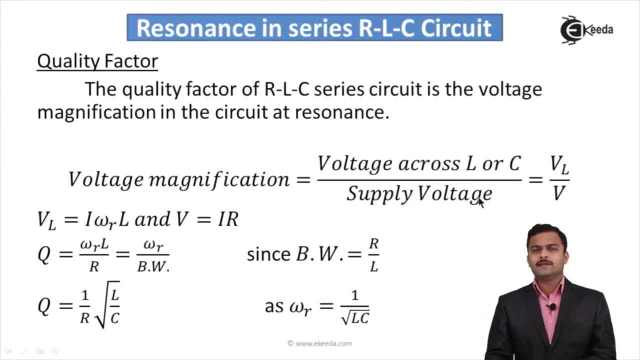 omega RL and supply voltage. everybody knows supply voltage is nothing but a voltage across resistance only. So if I substitute, I will get Q equal to omega RL divided by R, and R by L is nothing but a bandwidth. So this is one more formula for a quality factor, which is omega R divided by bandwidth. 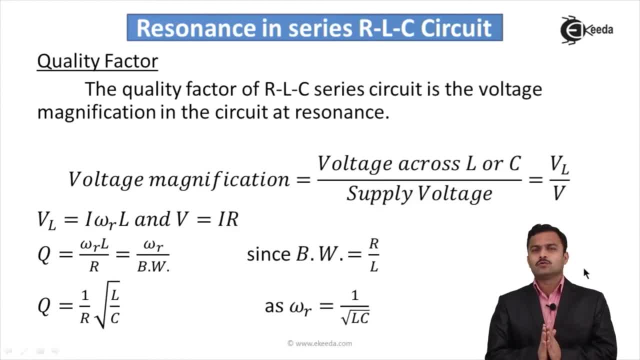 Omega R I will consider as 1 upon root of LC. So if I substitute 1 upon root of LC over here, what I will get? quality factor as 1 by R root of LC. So here I get a quality factor in terms of all the three passive elements. meaning if 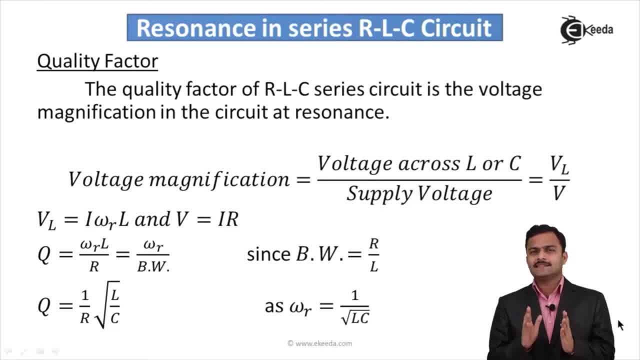 I know value of RLC, I can say what is the quality factor of the circuit. quality factor is nothing but that factor which will get multiplied to the supply voltage in order to get a voltage magnified value series. RLC circuit at resonance is also called as acceptor. 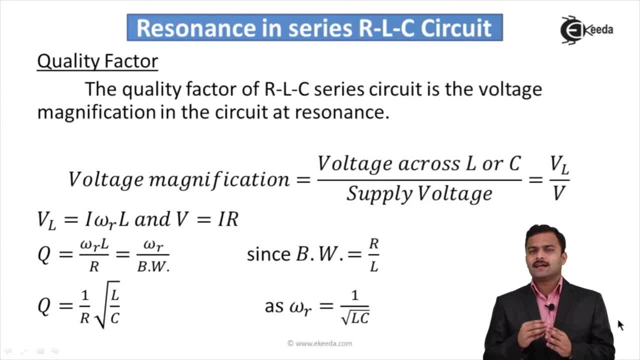 circuit. why? because at resonance current is maximum, so I can say current is getting accepted at a higher level at resonance. Therefore series RLC circuit at resonance is also called as acceptor circuit. So if I know the value of R, value of L, value of C, I can get so many parameters which are 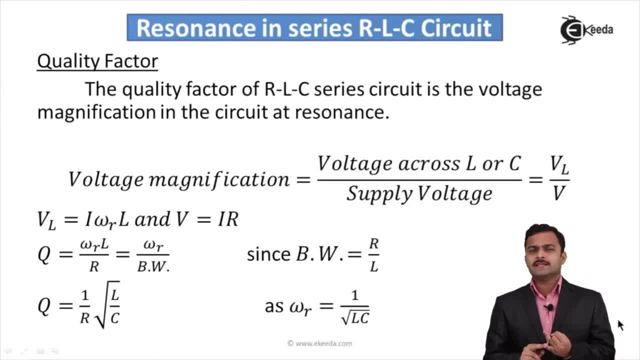 responsible for the resonance, Like resonating frequency, Bandwidth, lower cutoff frequency, higher cutoff frequency and quality factor of the circuit. so resonance is required in order to transfer maximum power from supply to the load.